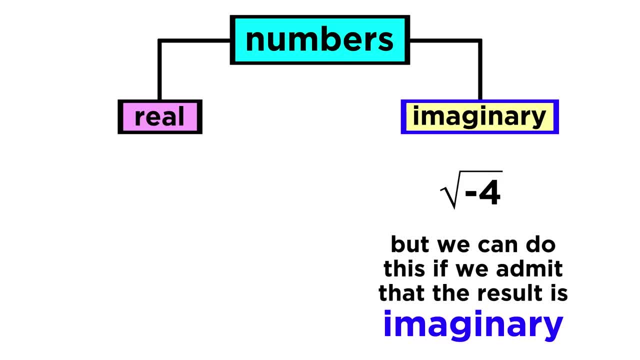 a negative number. However, in another sense, we can take the square root of a negative number if we admit that the result is imaginary, While the square root of one is simply one, we will say that the square root of negative one is I. This is a lowercase I, always in italics, and it is the fundamental imaginary. 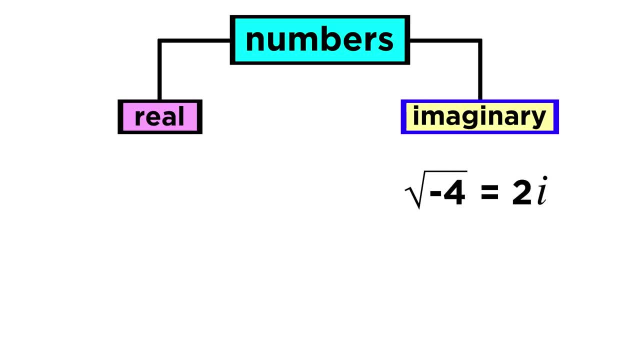 number. The square root of negative four would be two I, because negative four is equal to four times negative one. so this radical could be split up into root four times root negative one, which is therefore two times I or two I. That covers imaginary numbers, so let's go back to the real numbers. 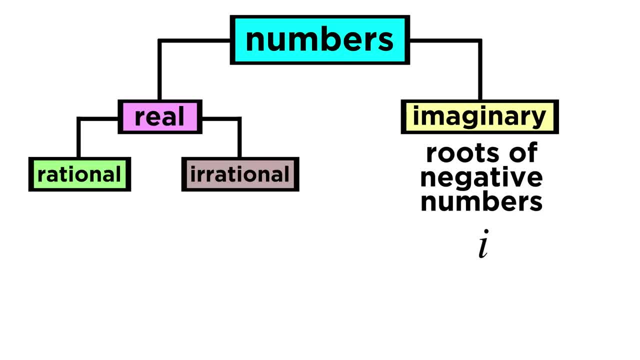 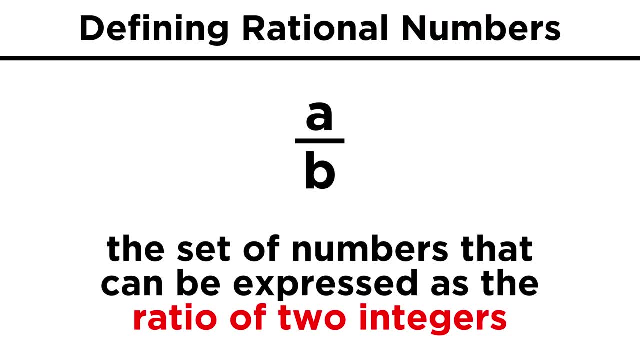 Within the category of real numbers, there are two subcategories: rational and irrational. Rational numbers are defined by the number of real numbers. Rational numbers are defined as any number that can be expressed as the ratio of two integers: Three halves, ninety-three, six hundred and fourths. you just make a fraction, put any. 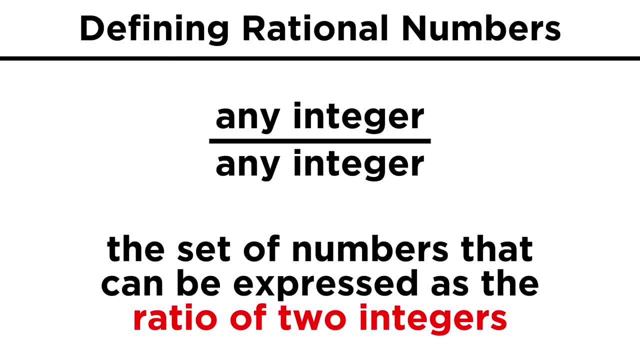 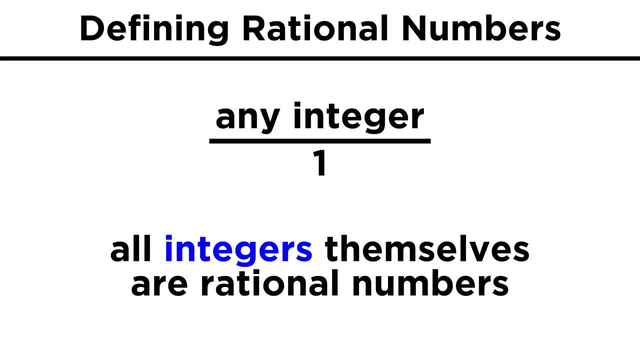 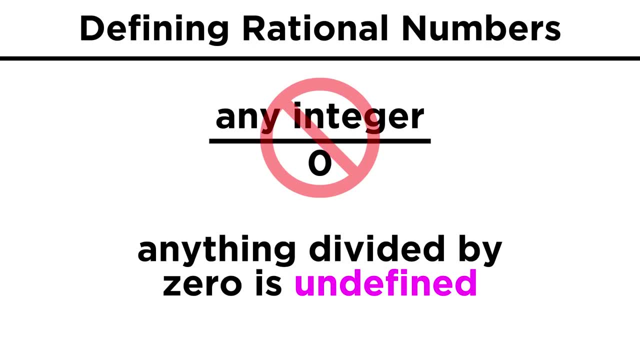 integer on top and any integer on the bottom, and you've got a rational number. The number on the bottom can also be one, so all the integers themselves qualify as rational numbers. The only number that can't go on the bottom is zero, as that will yield a value that is. 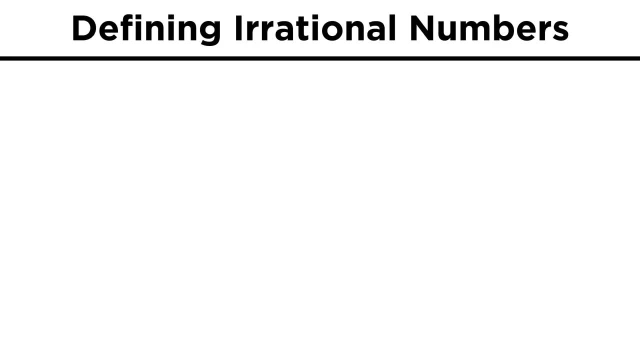 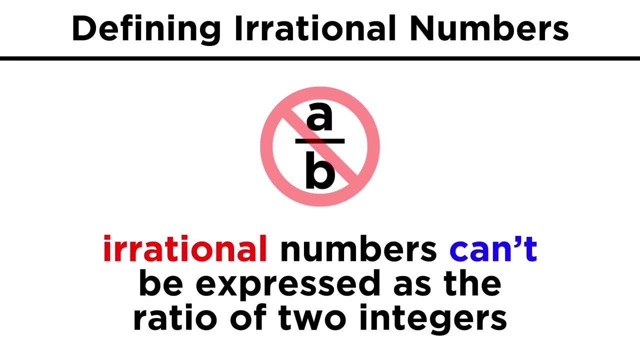 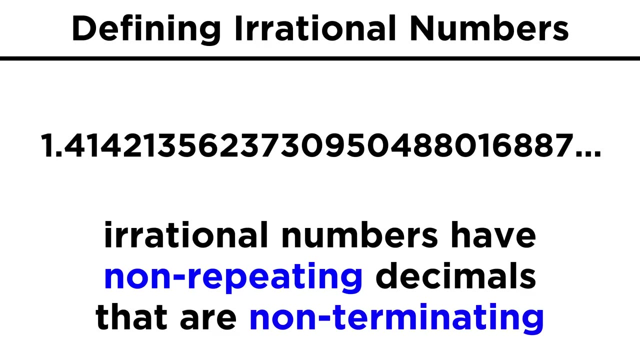 undefined. Now, what are these irrational numbers? Given the definition of a rational number, clearly an irrational number is one that can't be expressed as the ratio of two integers. But what could these numbers be? Irrational numbers are ones that have non-repeating decimals, that are non-terminating meaning. 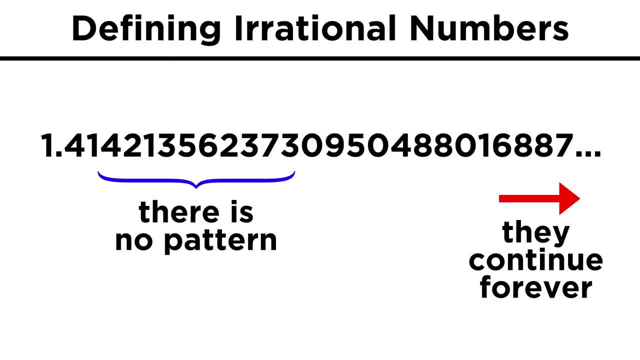 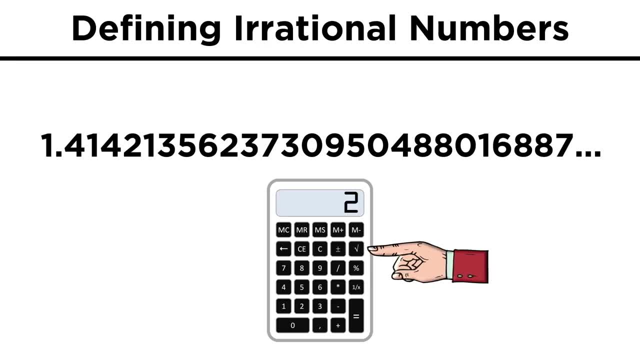 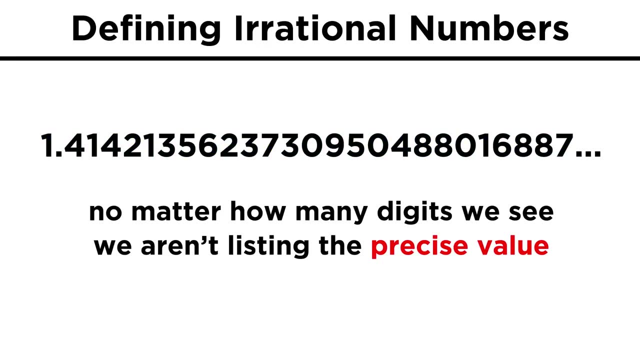 they continue forever with no pattern. The square root of two is such a number: If we plug this into a calculator, it will tell us that the answer is one point four, one, four, two, et cetera, et cetera. but no matter how many digits your calculator displays. 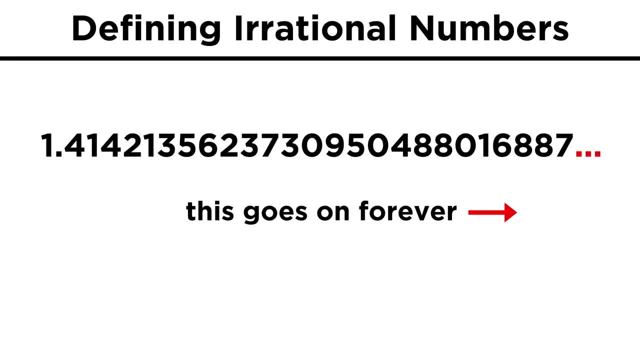 it's not giving you the full story. This number extends forever, which means we can never list the square root of two as a decibel and be infinitely accurate. the way we can, with three halves, Three halves or one point five is exactly three over exactly one. 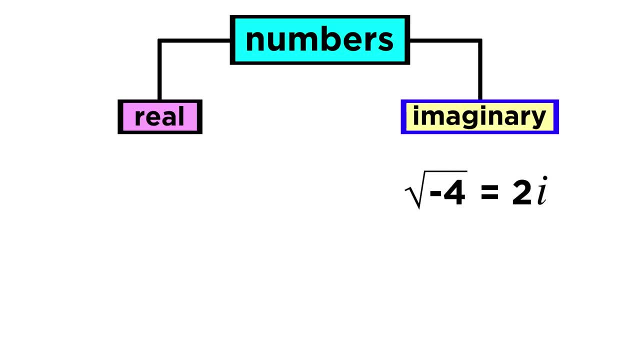 number. The square root of negative four would be two I, because negative four is equal to four times negative one. so this radical could be split up into root four times root negative one, which is therefore two times I or two I. That covers imaginary numbers, so let's go back to the real numbers. 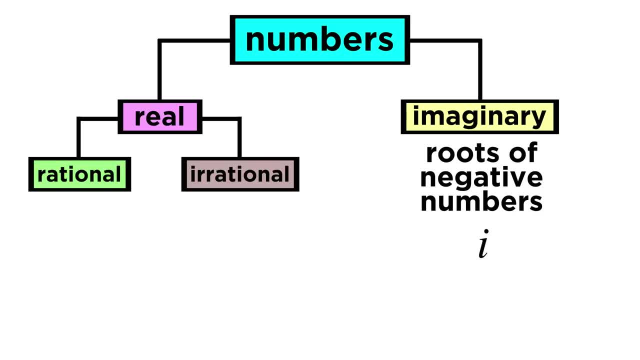 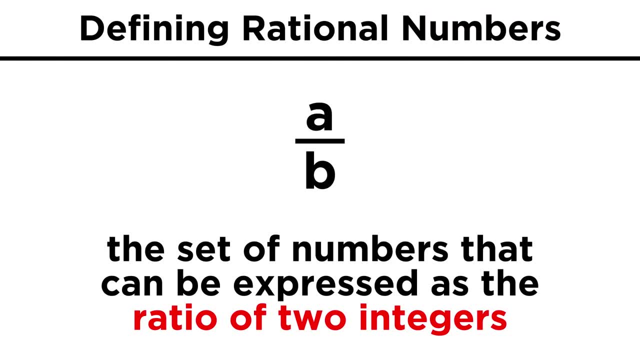 Within the category of real numbers, there are two subcategories: rational and irrational. Rational numbers are defined by the number of real numbers. Rational numbers are defined as any number that can be expressed as the ratio of two integers: Three halves, ninety-three, six hundred and fourths. you just make a fraction, put any. 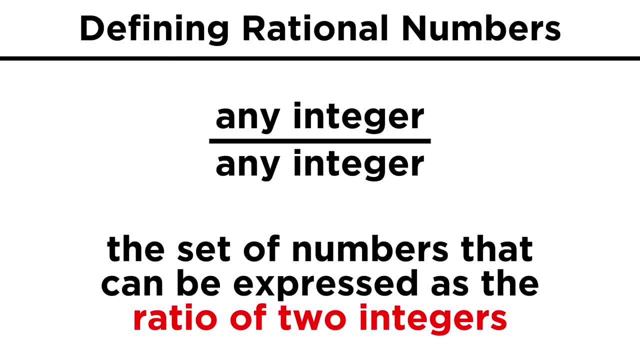 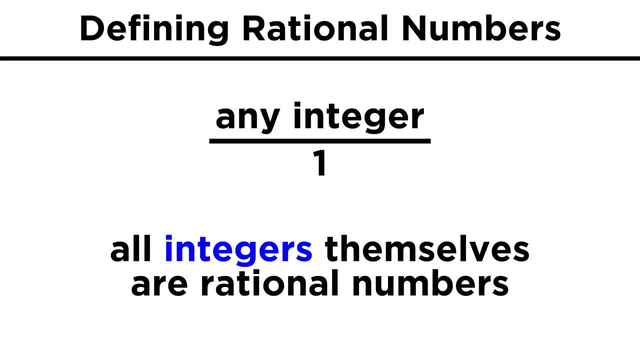 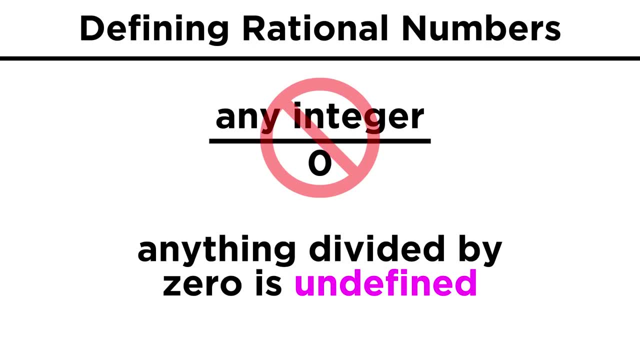 integer on top and any integer on the bottom, and you've got a rational number. The number on the bottom can also be one, so all the integers themselves qualify as rational numbers. The only number that can't go on the bottom is zero, as that will yield a value that is. 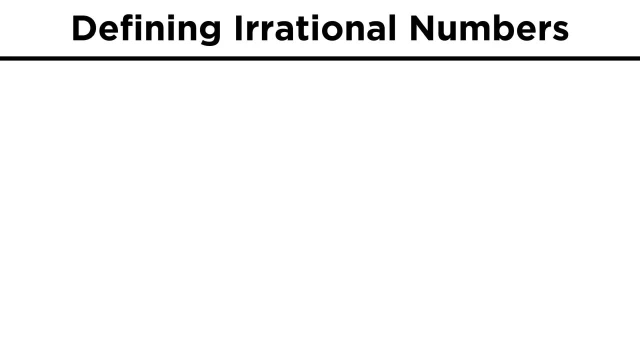 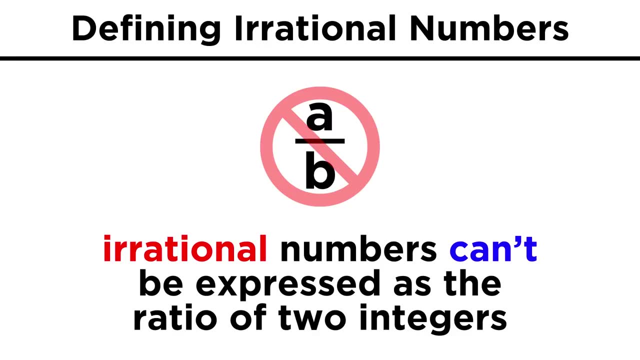 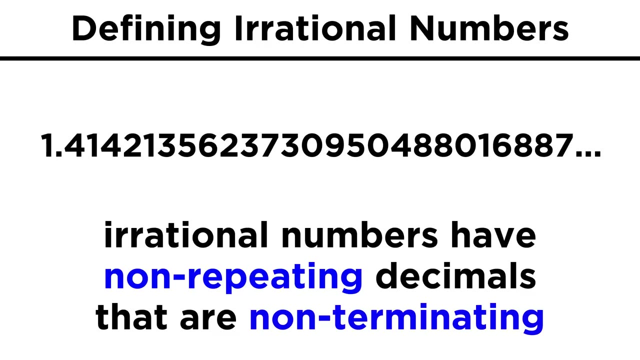 undefined. Now, what are these irrational numbers? Given the definition of a rational number, clearly an irrational number is one that can't be expressed as the ratio of two integers. But what could these numbers be? Irrational numbers are ones that have non-repeating decimals, that are non-terminating meaning. 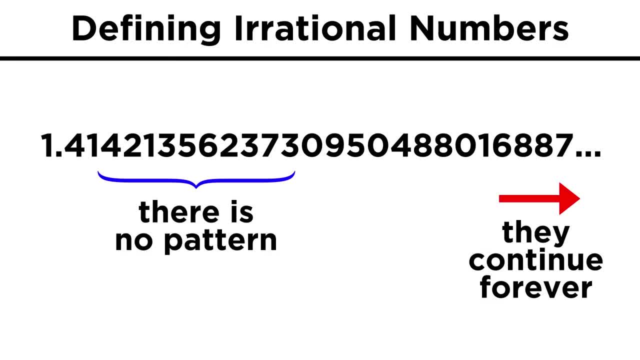 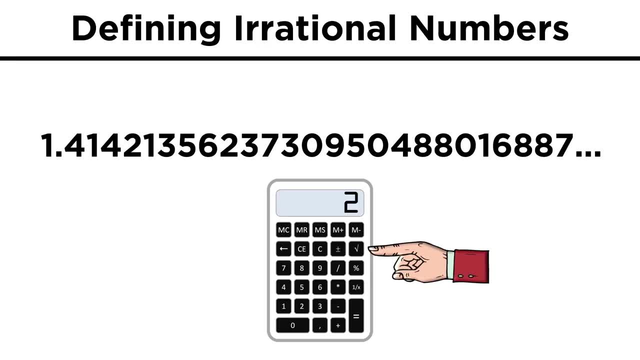 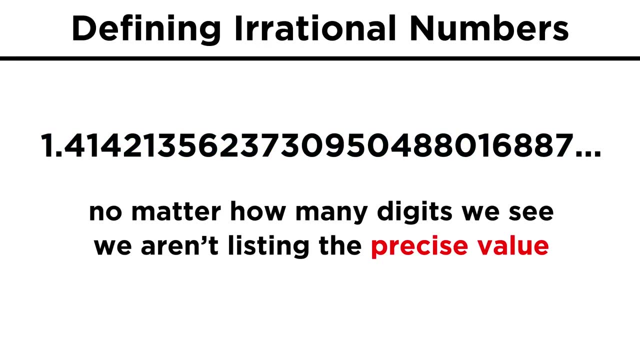 they continue forever with no pattern. The square root of two is such a number, It's not just a number. If we plug this into a calculator, it will tell us that the answer is one point four, one, four, two, et cetera, et cetera. but no matter how many digits your calculator displays, 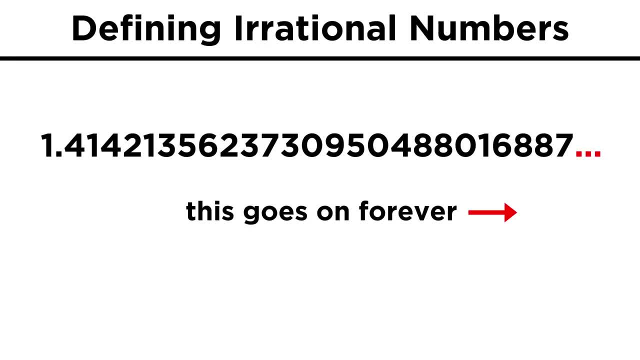 it's not giving you the full story. This number extends forever, which means we can never list the square root of two as a decibel and be infinitely accurate. the way we can, with three halves. Three halves or one point five is exactly three over a decimal. 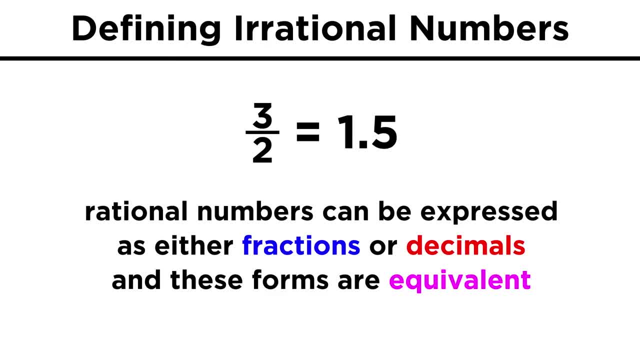 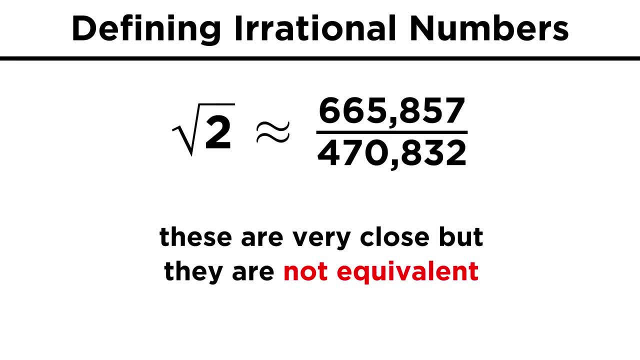 The answer is one point four, one, four, two, et cetera, et cetera, et cetera. If we try to approximate root two this way, we can get very close with something like six hundred sixty-five thousand, eight hundred fifty-seven over four hundred seventy thousand. 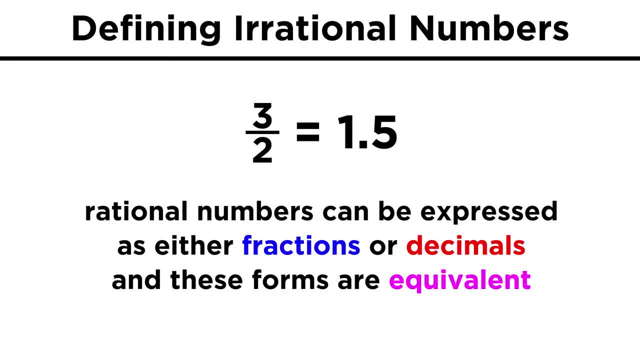 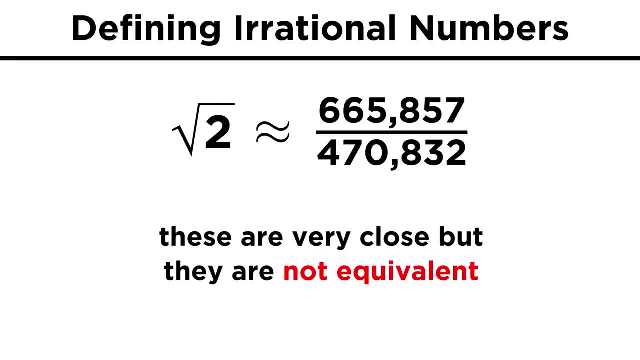 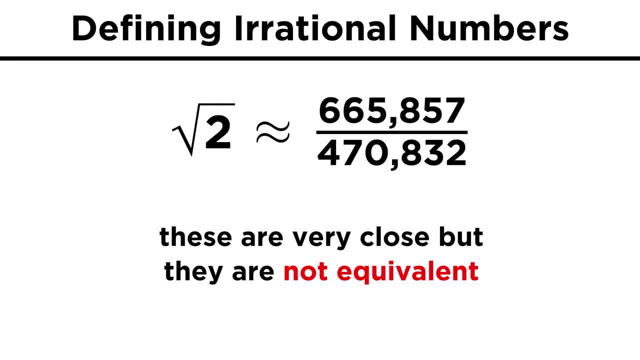 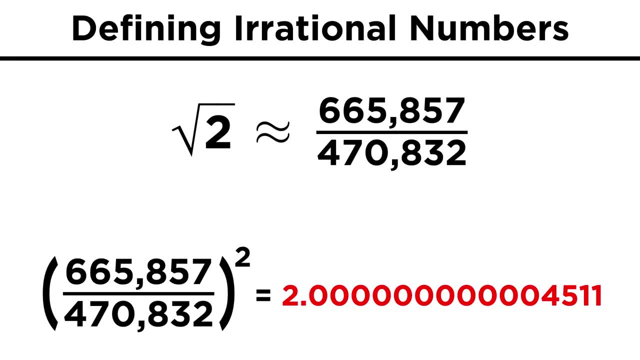 eight hundred thirty-two, But it's not exactly right. and when we square this number, we get something just ever so slightly larger than two. No matter how precise you try to get with this ratio, you will never quite get to the true value. 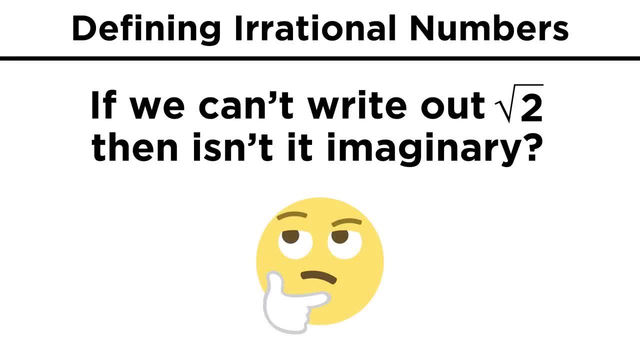 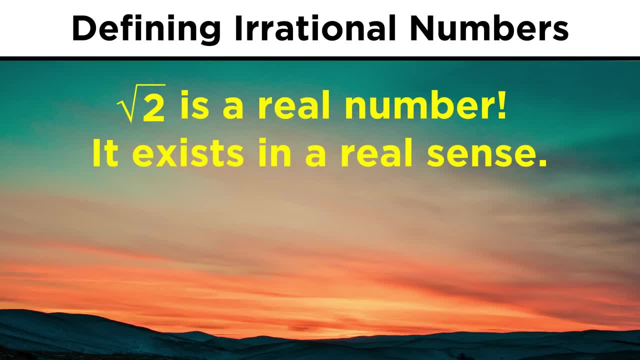 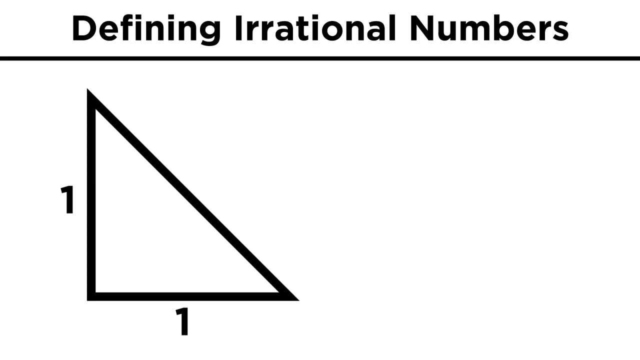 Now you might be wondering if we can't write out this number. no matter what we do, doesn't that make this number imaginary? The answer is no. Nature is very clear in communicating to us that numbers like root two do indeed exist. 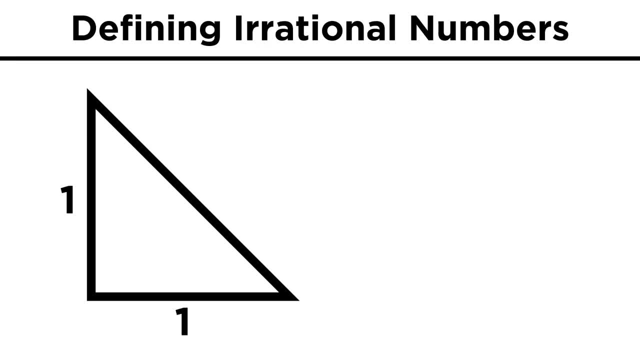 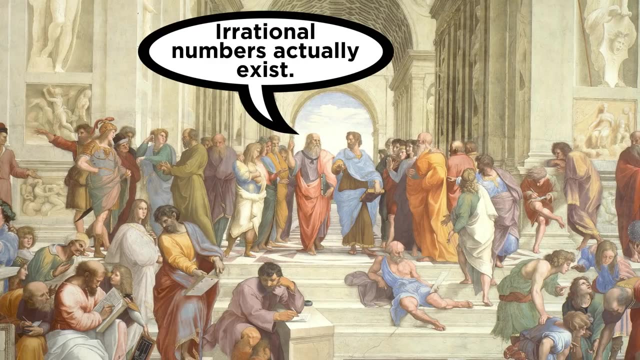 If you make a right triangle that has legs with a length of one, the third side will have a length of root two. This triangle exists, so root two exists. It is a real number. It's simply irrational. When it was discovered by the ancient Greeks that irrational numbers must exist, all hell. 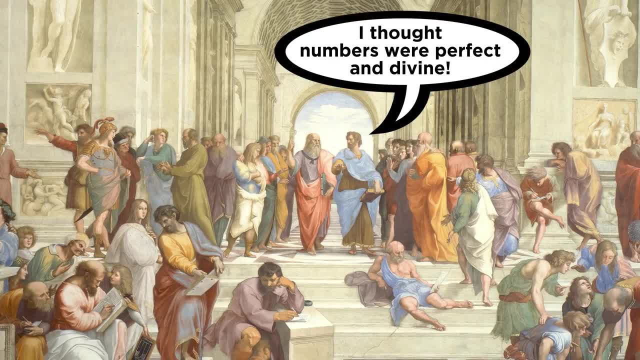 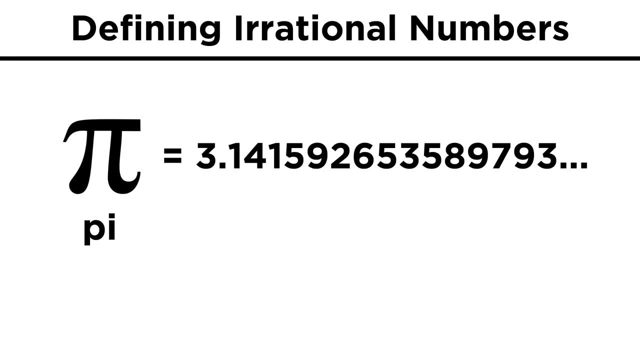 broke loose as it threatened the mystical notion that the world of numbers must obey a divine perfection. Other irrational numbers include pi, which is the ratio of the circumference of a circle to its diameter. We all probably know the first few digits of pi, which are three point one, four, one. 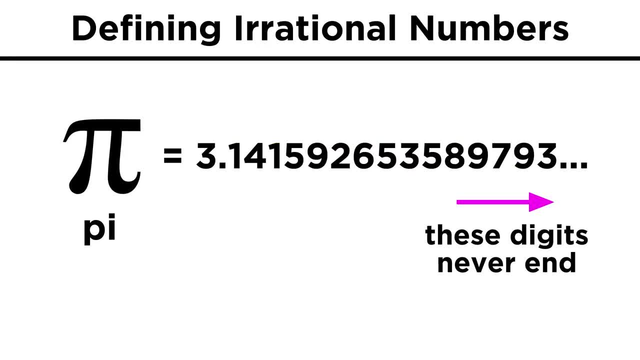 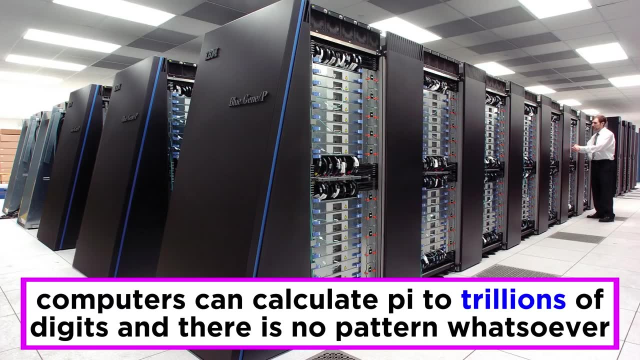 five, nine, yadda, yadda, yadda Again. this number never ends with no pattern whatsoever in the digits. And it's not for lack of trying mathematicians have checked. With computers, we can calculate pi out to literally trillions of decimal places. and 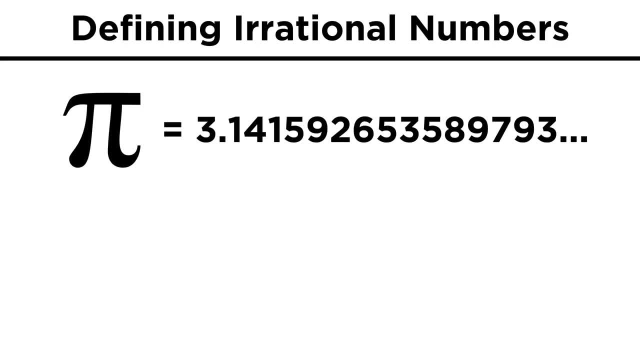 the numbers are random throughout. Once again, even though pi is irrational, it is a real number because circles are real and all circles have a circumference. But we will get to triangles and circles when we start looking at geometry right after this. 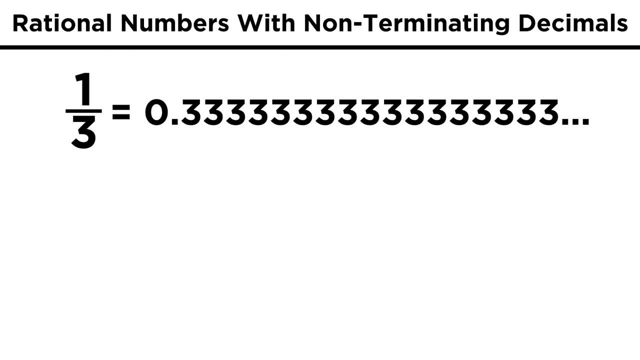 Let's quickly mention that there are numbers with non-terminating decimals that are actually rational. Take, for example, one third. If we convert this to a decimal, we get zero point three, with the three repeating forever, Although the threes go forever. this is a pattern. 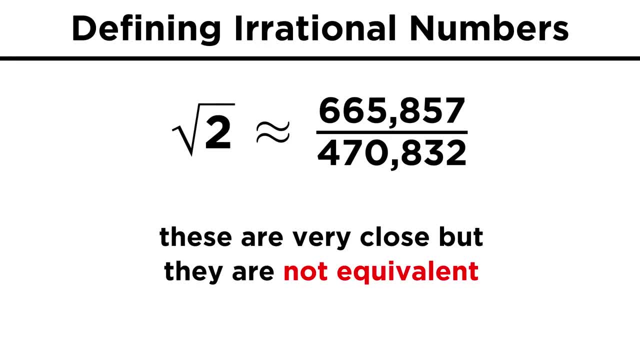 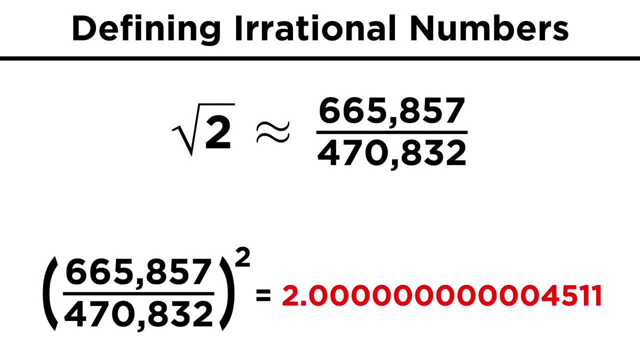 eight hundred thirty-two, But it's not exactly right. and when we square this number, we get something just ever so slightly larger than two. No matter how precise you try to get with this ratio, you will never quite get to a two. 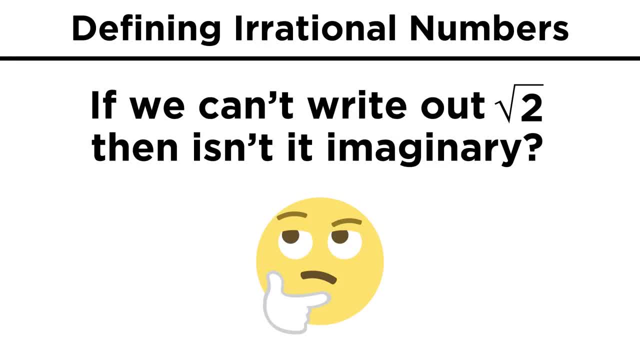 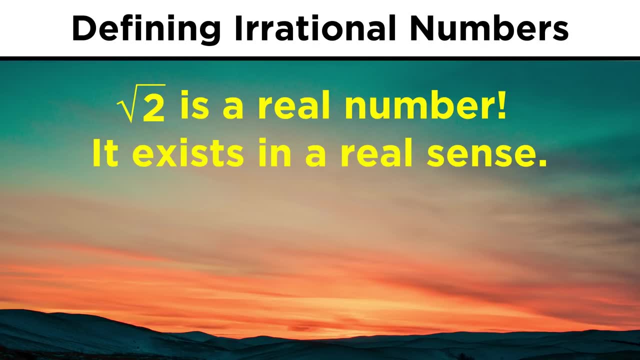 Now you might be wondering if we can't write out this number. no matter what we do, doesn't that make this number imaginary? The answer is no. Nature is very clear in communicating to us that numbers like root two do indeed exist. 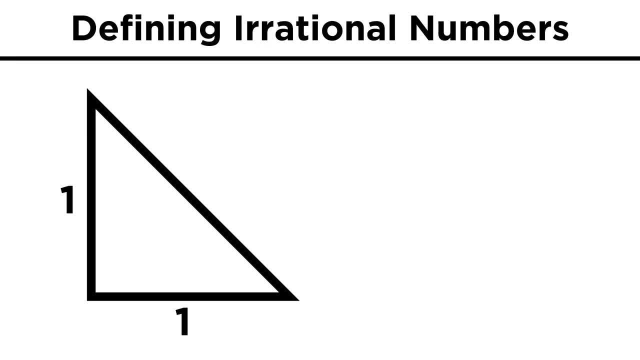 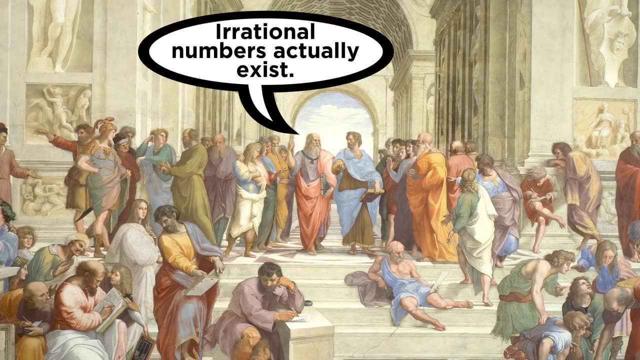 If you make a right triangle that has legs with a length of one, the third side will have a length of root two. This triangle exists, so root two exists. It is a real number. it is simply irrational. When it was discovered by the ancient Greeks that irrational numbers must exist, all hell. 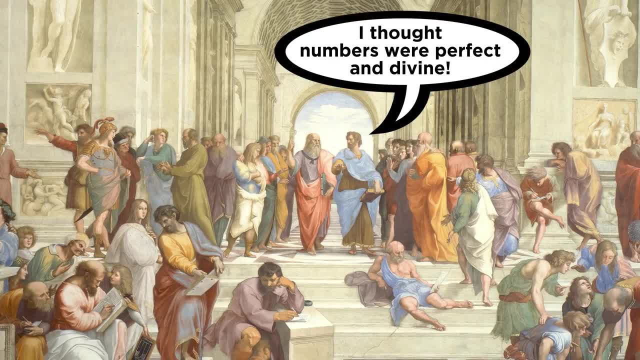 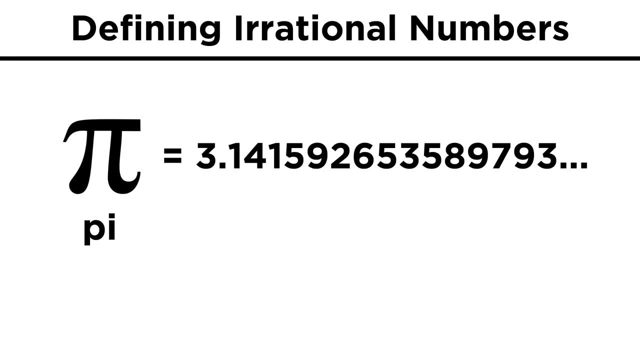 broke loose as it threatened the mystical notion that the world of numbers must obey a divine perfection. Other irrational numbers include pi, which is the ratio of the circumference of a circle to its diameter. We all probably know the first few digits of pi, which are three point one, four, one. 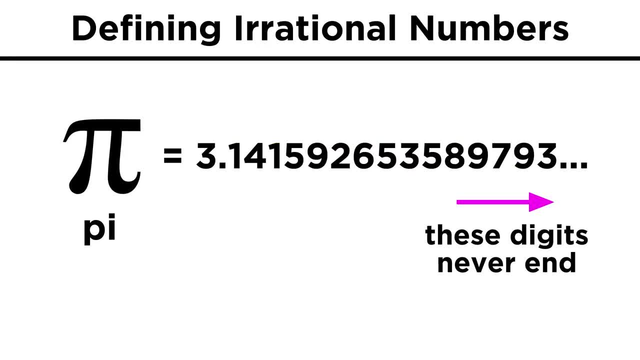 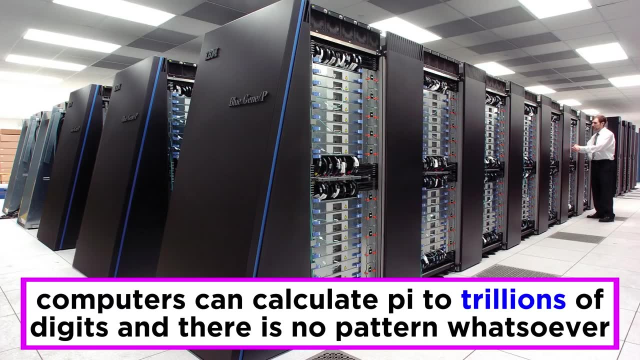 five and a half Five, nine, yadda, yadda, yadda Again. this number never ends with no pattern whatsoever in the digits. And it's not for lack of trying. mathematicians have checked. With computers we can calculate pi out to literally trillions of decimal places. and 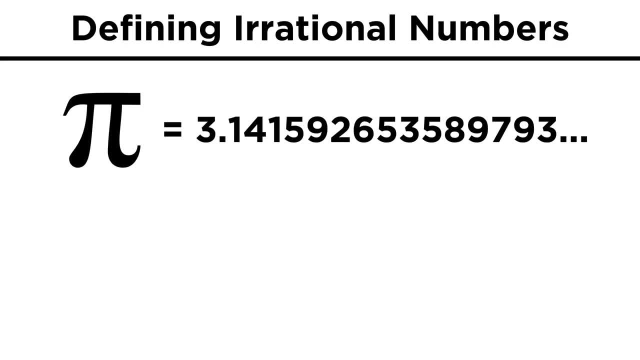 the numbers are random throughout. Once again, even though pi is irrational, it is a real number because circles are real and all circles have a circumference. But we will get to triangles and circles when we start looking at geometry right after this. 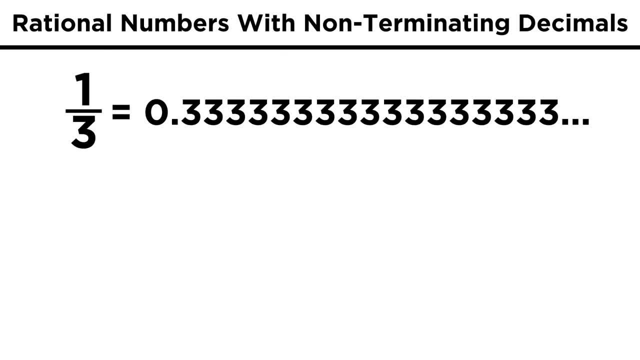 Let's quickly mention that there are numbers with non-terminating decimals that are actually rational. Take, for example, one third. If we convert this to a decimal, we get zero point three, with the three repeating forever, Although the threes go forever. this is a pattern. 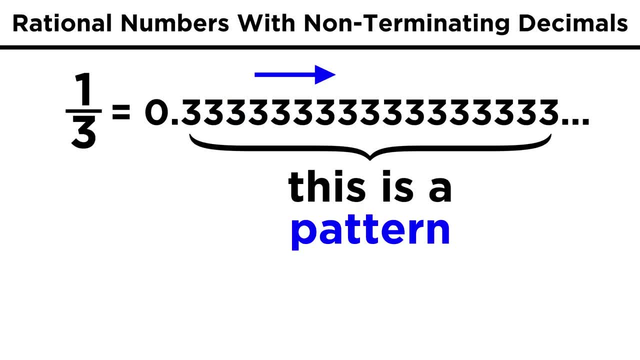 It's three, then three, then three and so forth, When decimals extend forever. but in a pattern like this they are actually rational, because they can indeed be expressed as the ratio of two integers, In this case one over three. 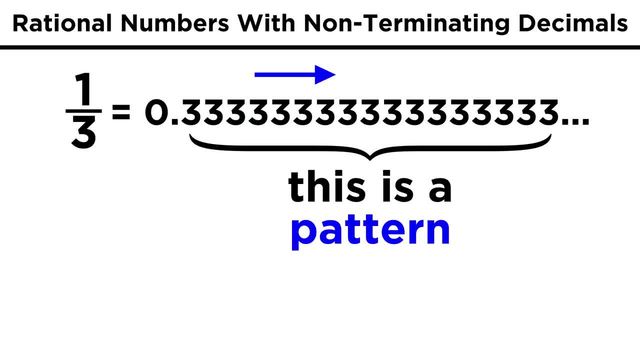 It's three, then three, then three and so forth, When decimals extend forever. but in a pattern like this they are actually rational, because they can indeed be expressed as the ratio of two integers, in this case one over three. 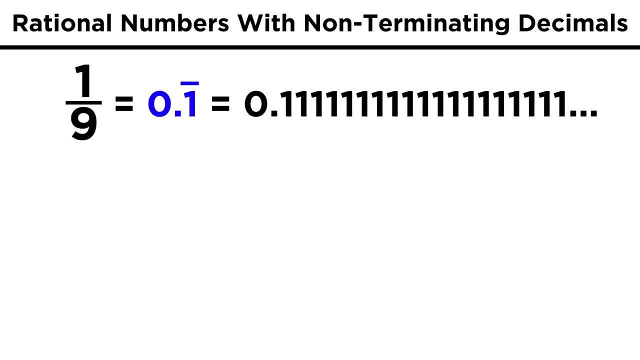 Another example would be one, ninth or zero point one, repeating. That's what this little bar means. whatever is under the bar repeats forever. in this case, just the number one. Two ninths is equal to zero point two, repeating. And this continues all the way up to nine. 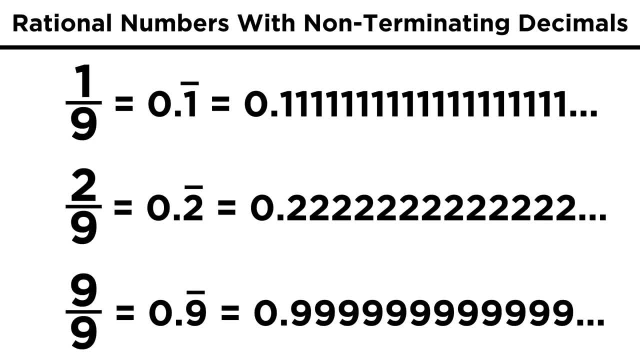 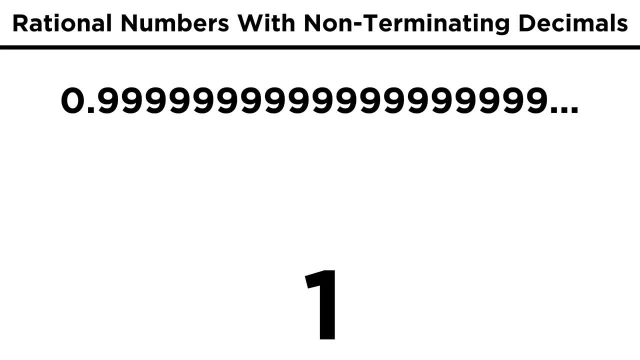 Nine, ninths, That would be zero point nine repeating, and this is absolutely equivalent to one. To prove this, we can rationalize that if the nines extend forever, then there cannot be any number in between this number and one, and they therefore must be the same number. 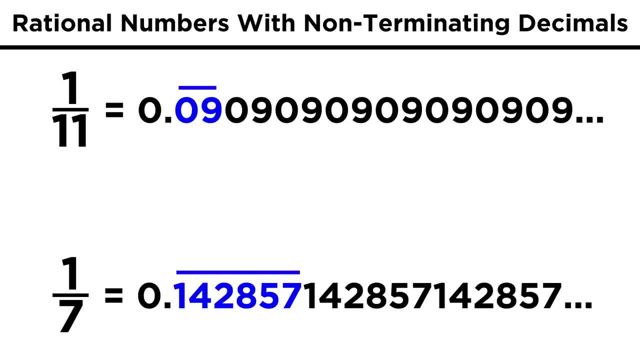 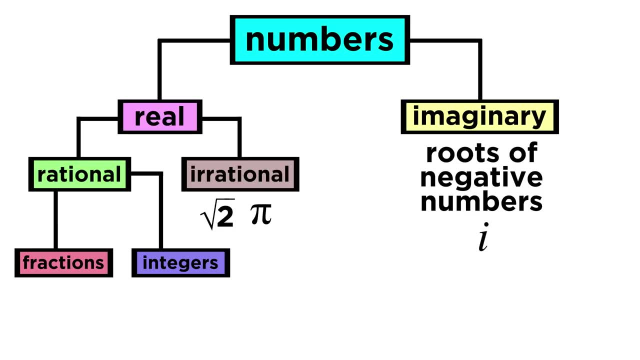 There are other numbers with non-terminating decimals in a pattern of two or three repeating digits or more. Let's look at some rational numbers that are simply the decimal versions of some fraction. If we want to, we can subdivide rational numbers further to describe types of numbers we already 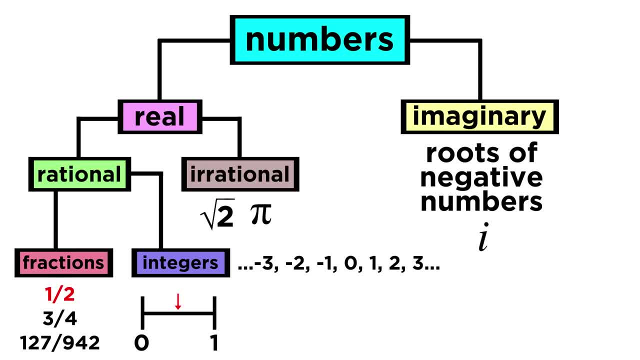 know about, like fractions and integers. Fractions are all the numbers that happen in between the integers, and there are infinitely many of them in between each integer. Within integers, we can describe whole numbers, which are all the integers, starting from one. 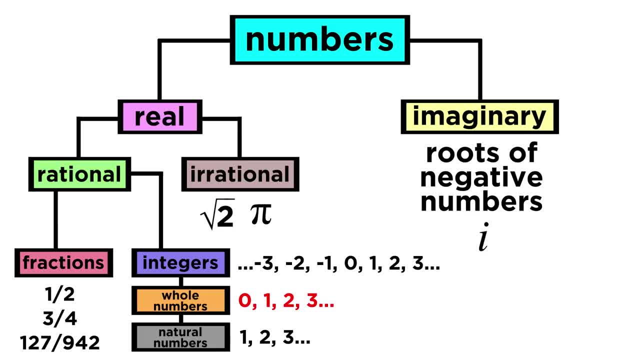 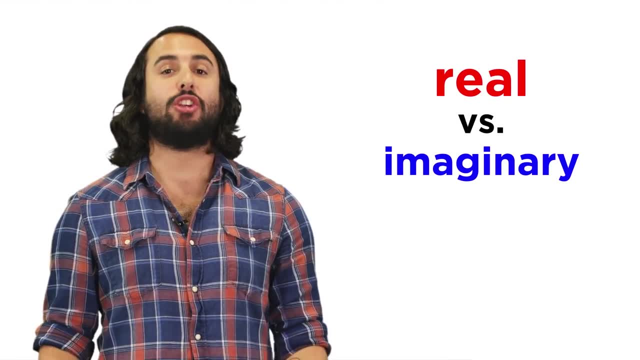 starting from zero and going in the positive direction, and natural numbers, which are all the integers starting from one, so the same as whole numbers, just without the zero. And that's pretty much all we need. After all this, we should be able to describe the difference between real and imaginary. 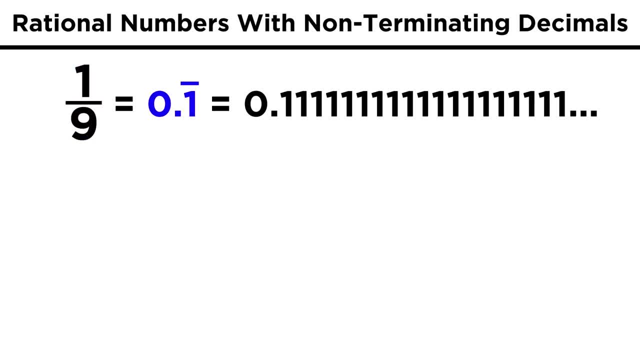 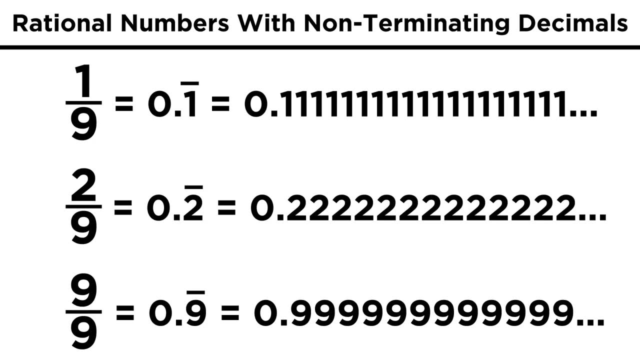 Another example would be one, ninth or zero point one, repeating. That's what this little bar means. whatever is under the bar repeats forever. in this case, just the number one. Two ninths is equal to zero point two, repeating. And this continues all the way up to nine ninths. 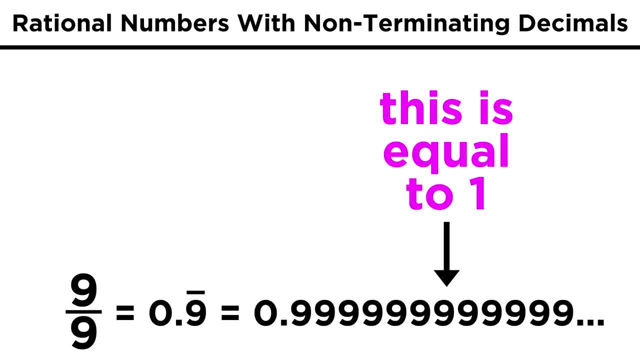 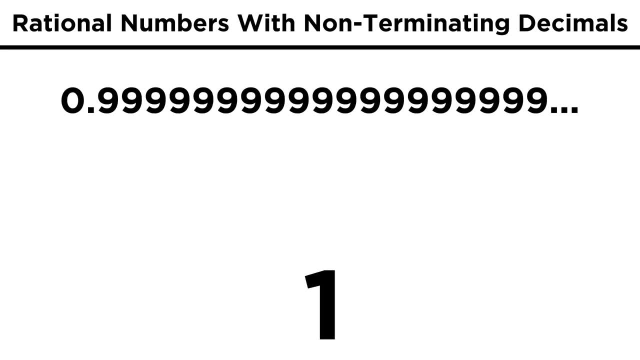 That would be zero point nine repeating, and this is absolutely equivalent to one. To prove this, we can rationalize that if the nines extend forever, then there cannot be any number in between this number and one, and they therefore must be the same number. 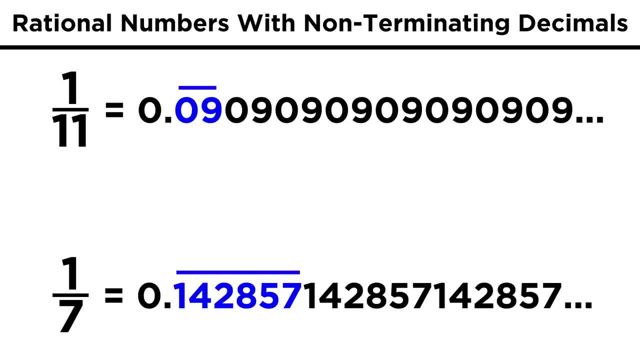 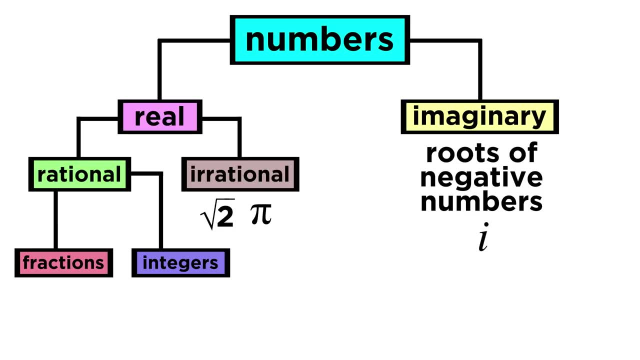 There are other numbers with non-terminating decimals in a pattern of two or three repeating digits or more. These are all rational numbers that are simply the decimal versions of some fraction. If we want to, we can subdivide rational numbers further to describe types of numbers we already 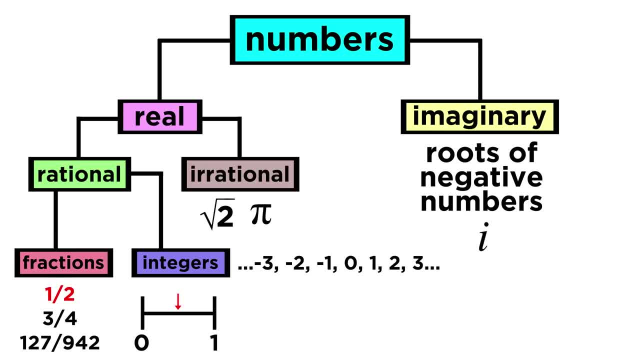 know about, like fractions and integers. Fractions are all the numbers that happen in between the integers, and there are infinitely many of them in between each integer. Within integers, we can describe whole numbers, Whole numbers, which are all the integers starting from zero and going in the positive. 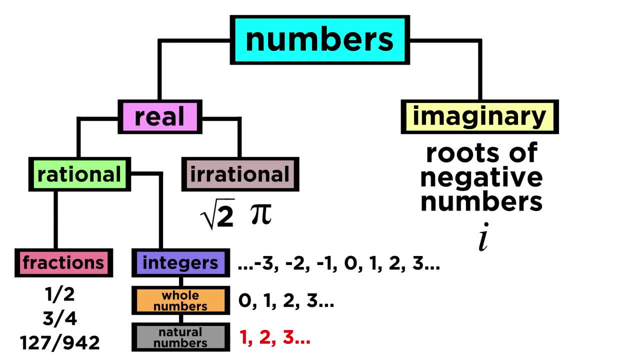 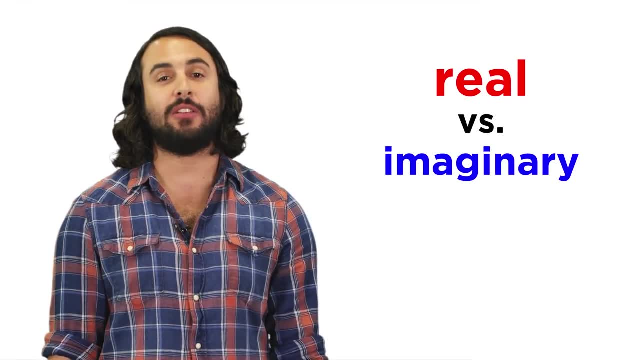 direction, and natural numbers, which are all the integers starting from one, so the same as whole numbers, just without the zero. And that's pretty much all we need. After all this. we should be able to describe the difference between real and imaginary. 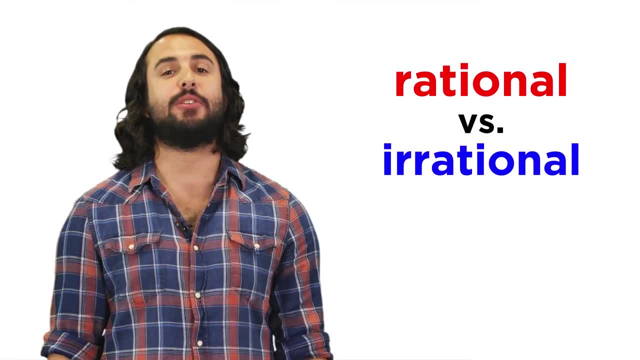 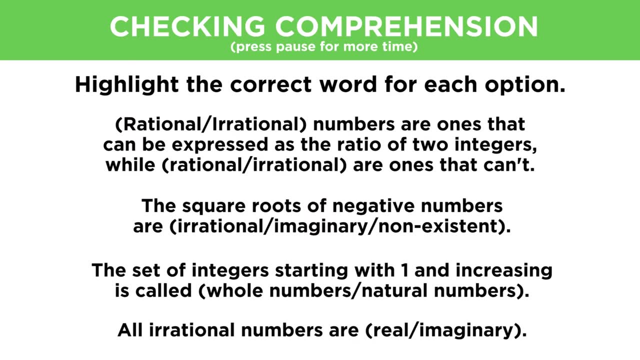 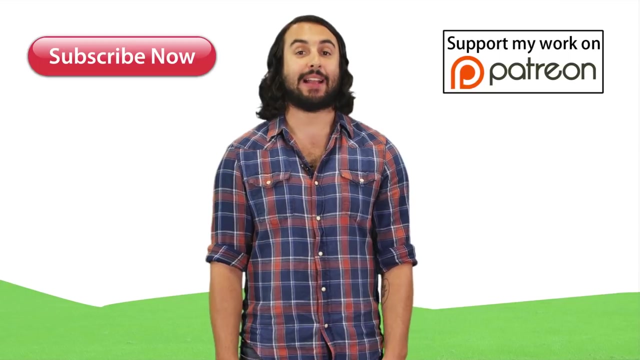 numbers and, within the real numbers, the difference between rational and intangible Irrational numbers. To make sure that's the case, let's check comprehension. Thanks for watching, guys. Subscribe to my channel for more tutorials. support me on patreon so I can keep making.